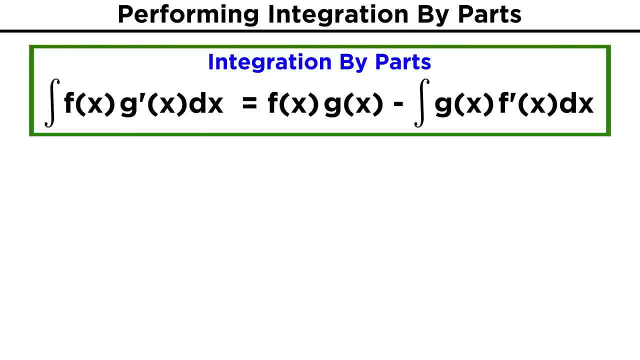 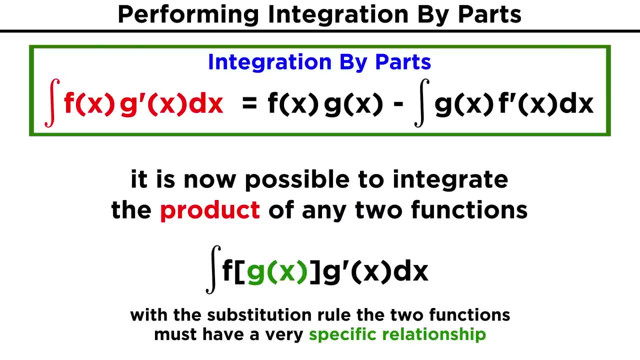 It may look like we haven't done much, but this is actually quite powerful, because up until now we haven't had any way to integrate a product of two functions other than the substitution rule, if we were lucky enough that one part was the derivative of the other. 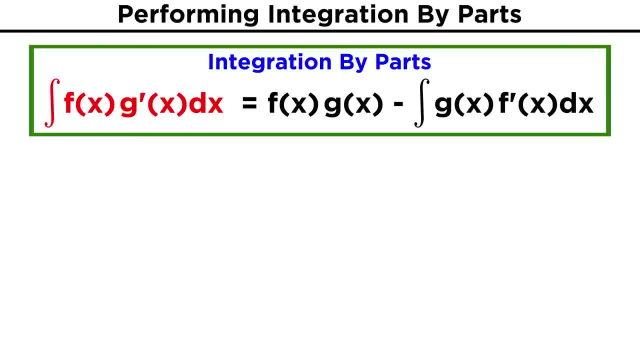 But here we can see that if we have the product of two functions to integrate, we simply list the first function times the antiderivative of the second function, since the antiderivative prime is simply g, and subtract from that the integral of the antiderivative of the. 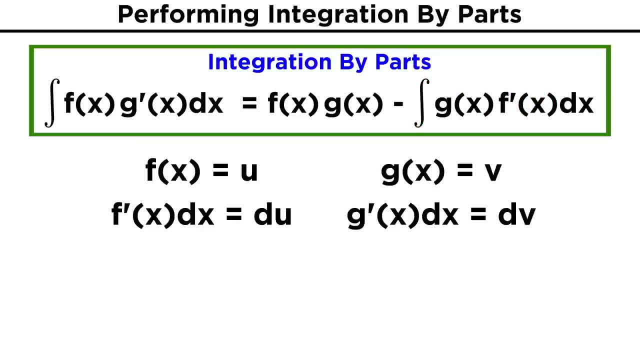 second function times the derivative of the first function. An easier way to remember all of this is to represent f of x as u and g of x as v. Then the first integral becomes u, dv, and then we have uv minus the integral of v, du. 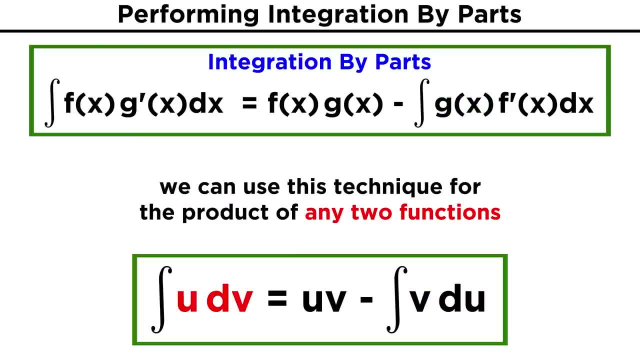 The thing to keep in mind here is that, while we can apply the technique to any integrand that is a product of functions, sometimes this will make things simpler and sometimes it won't- You'll notice that the technique leaves us with a different integral to evaluate. 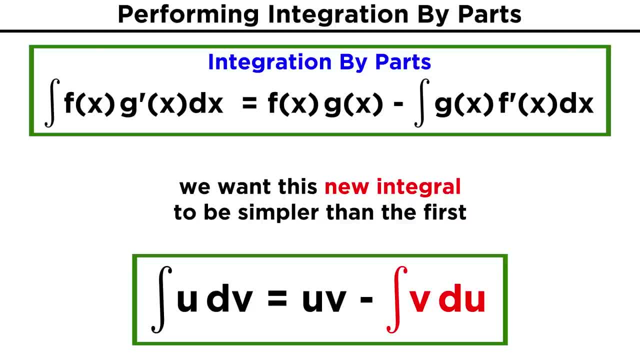 and if this one is no simpler than what we started with, then this technique is not very useful. But let's look at some examples where this approach works like a charm and you'll get a better sense of exactly what we're doing. Let's look at some examples where this approach works like a charm and you'll get a better sense of exactly what we're doing. 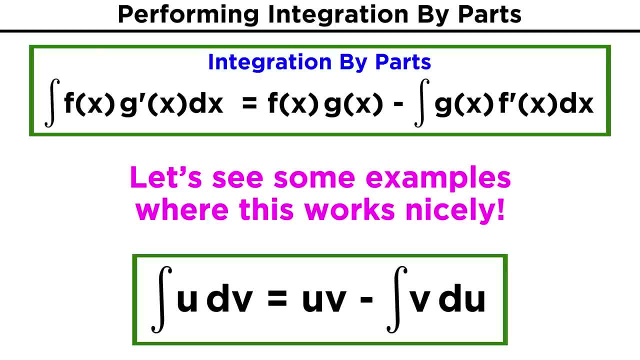 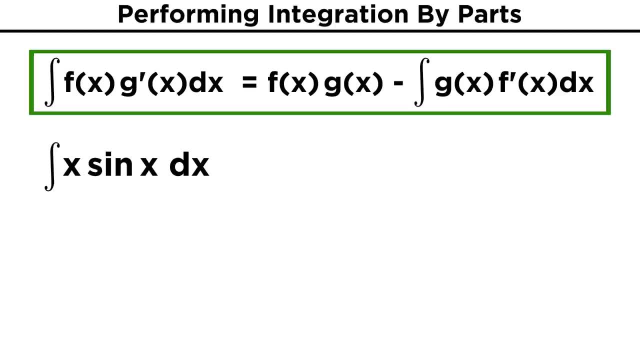 Let's try to integrate x sine x, dx. Before we start getting used to u's and v's, let's just use the first formula with f and g. Here's a hint. We know that between these two functions x and sine x. one of them will be f and the 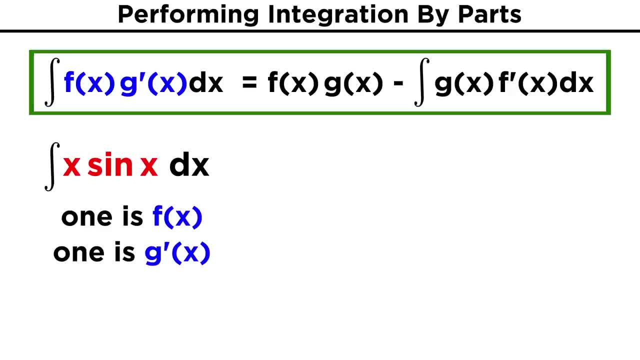 other will be g prime. The trick is that we want the function that becomes much simpler when differentiated to be f, because f prime will remain in the integral over here and we will want to be able to evaluate this integral easily. so let's use x as f of x, because its derivative 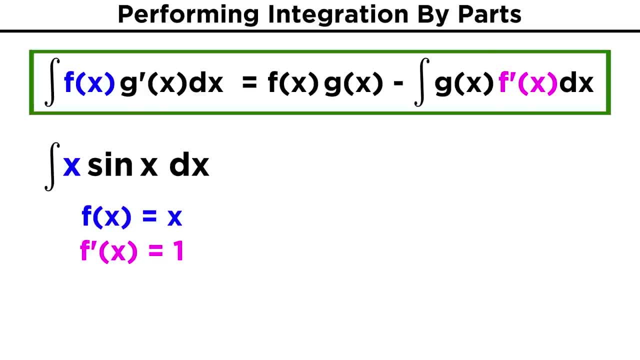 is one which is as simple as it gets. So in the first integral, x will be f of x and sine x will be g prime of x. Then, to see what this integral is equal to, the first term will be f of x and sine x. 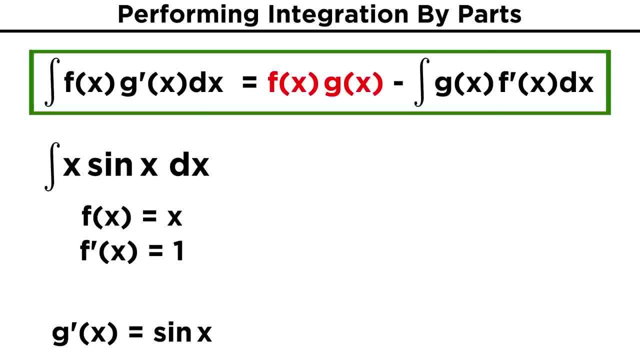 will be g prime of x. The second term will be f of x times g of x. so it's x times the antiderivative of sine x, which we know is negative cosine x. So that's negative x cosine x. Now to evaluate the other integral. 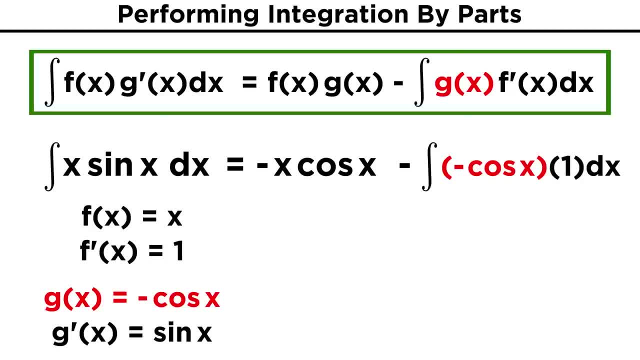 We know that g of x is negative cosine x, as we just said. But here's the best part: f prime of x is one. so this second integral is simply negative cosine x. We can take out the negative sign to cancel out the first one. 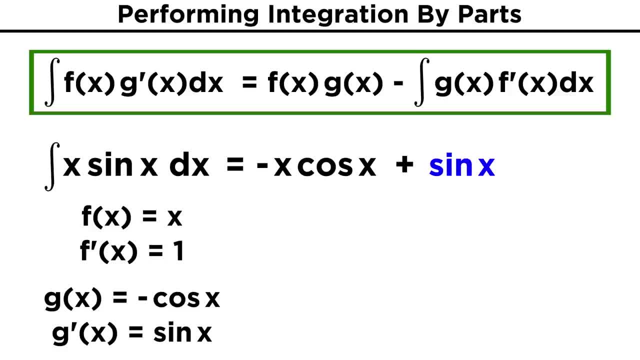 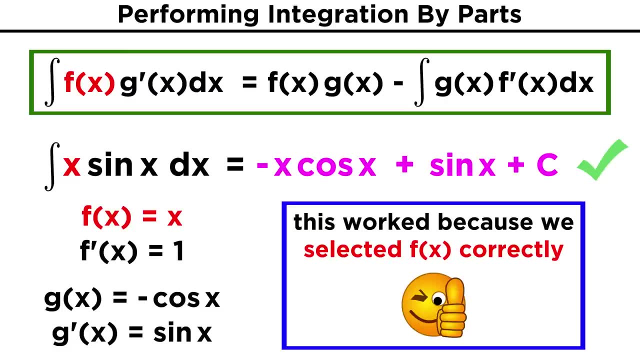 Cosine x is trivial to integrate. It's sine x. So we are left with negative x cosine x plus sine x plus c. So bear in mind that the reason this worked is because we chose the function for f of x. that would yield an f prime function. that would make this second integral much simpler. 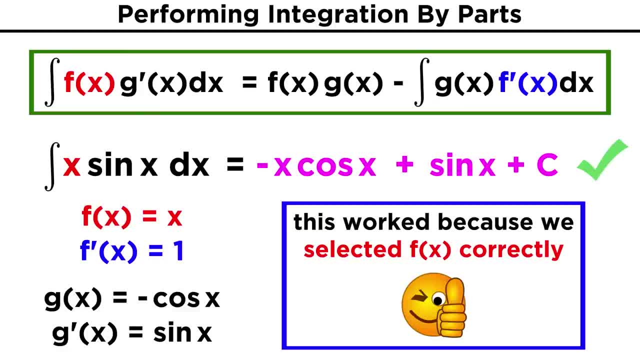 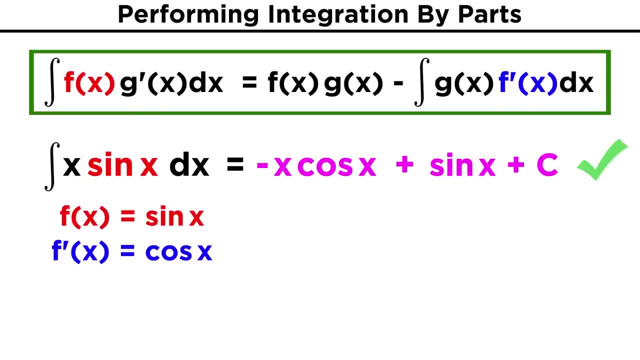 Much easier to evaluate than the first. In this case that was x, because its derivative is one. Choosing sine x would have been a bad idea because its derivative is just another trig function, cosine, and the other integral wouldn't have been any easier to evaluate. so this: 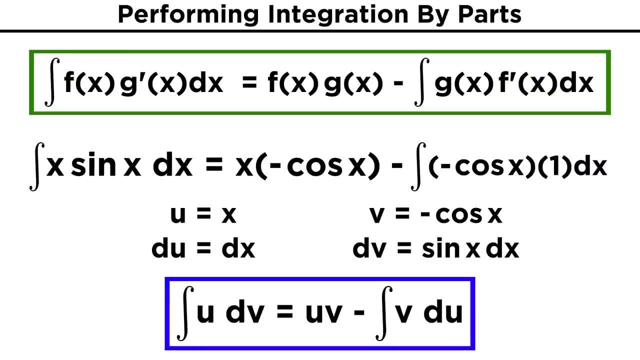 method wouldn't work. Let's now just explain the other notation we will have to learn using the same example. We could also have written this with a u in the first integral instead of x. So we could have written this with a u in the first integral instead of x. 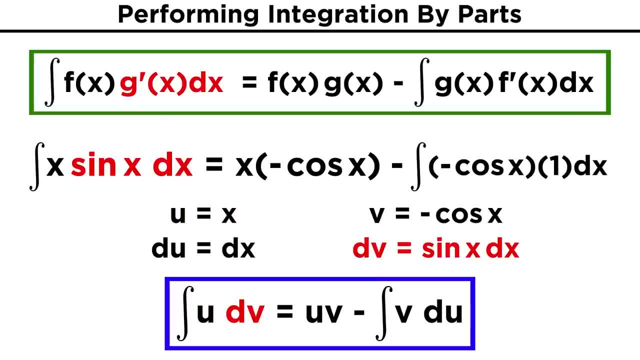 So we could have written this with a u in the first integral instead of x, And then dv instead of sine x, dx. That's because dv is the derivative of v, which is the g of x. that was found by taking the antiderivative. 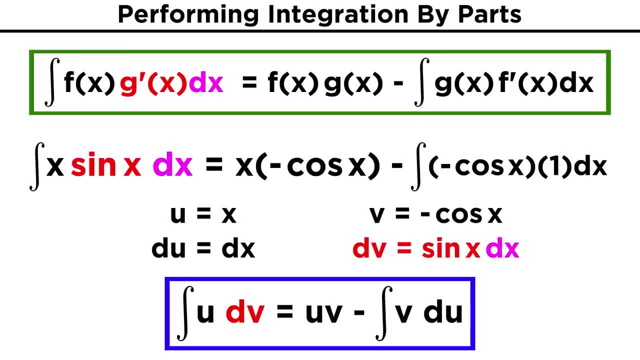 So always make sure the dx is part of the dv. Then this ended up equaling uv minus the integral of vdu. The reason this is useful is because if we set up these relationships for which function represents what? Then we can just write out the answer this simpler way and plug everything back in according. 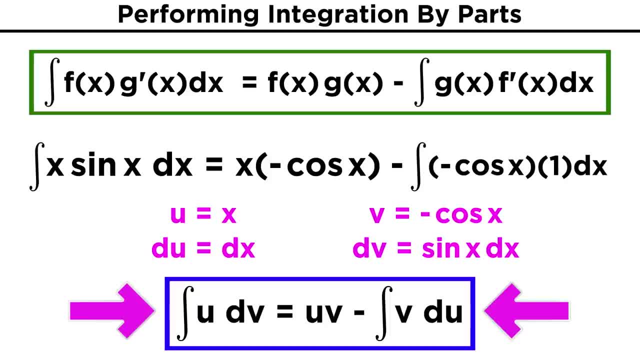 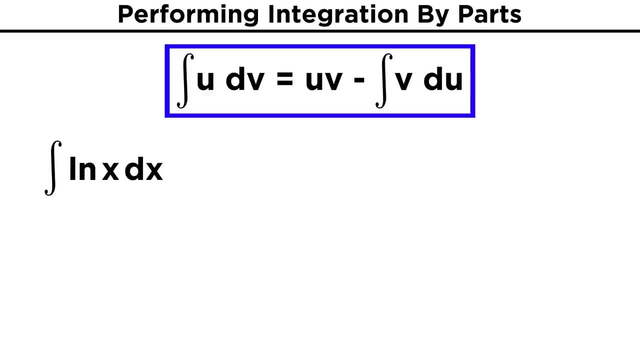 to our assignments to evaluate. Let's try another and you'll see what I mean. Say we want to integrate the natural log of x- dx. This is not a common integral and it also doesn't appear to be a product. but let's 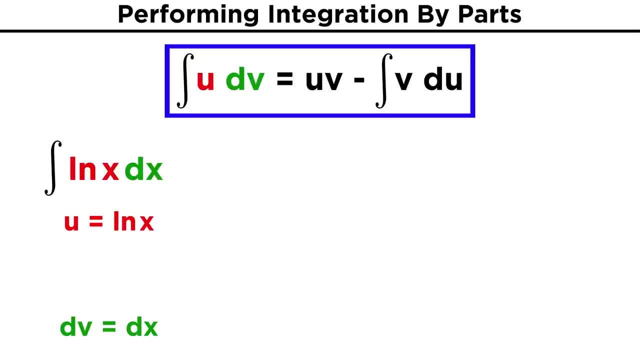 see how we actually can integrate by parts. We have to assign u and dv first, And here there is only one option, as the integral is the integral of u, And here there is only one option as the integral of u and dv. 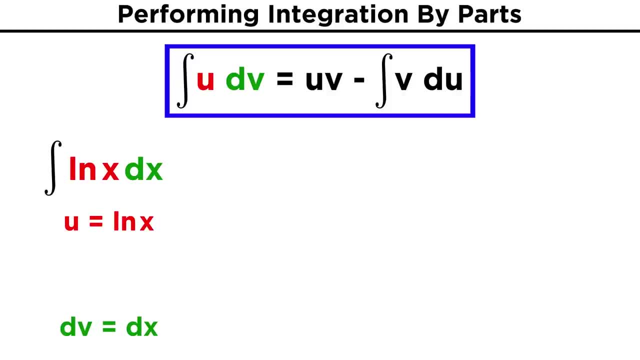 And here there is only one option as the integral of u and dv. And here there is only one option as the integral of u and dv. And here there is only one function: Natural log of x will become u and dx will become dv. 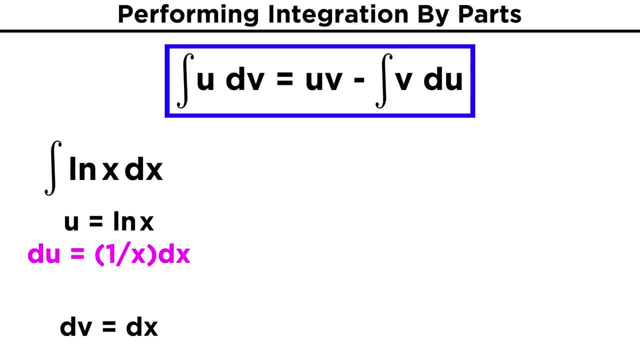 When we write out the answer, we will also need du, which is the derivative of u, and that's one over x, dx, And we need v, which is the antiderivative of dv. so from dx we get x. Now we just use the formula. 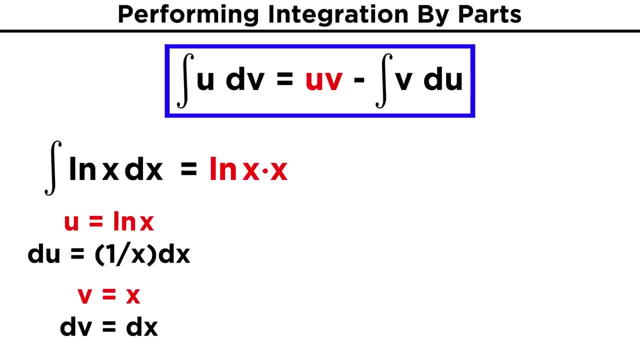 The product uv will be the natural log of x times x or xlnx. Then we subtract from that the integral of vdu. V is x and du is one over x, dx. so the x's cancel, leaving us with simply dx. 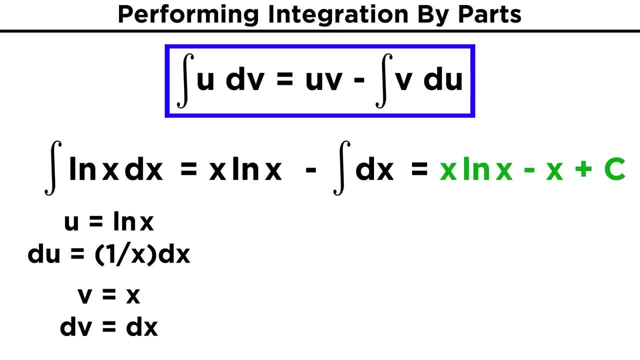 Integrating dx gives us x and our final answer is xlnx minus x plus c. So once again, we took an integral that we couldn't eventuate. So once again, we took an integral that we couldn't eventuate And turned it into a different expression with a different integral in it. that happened. 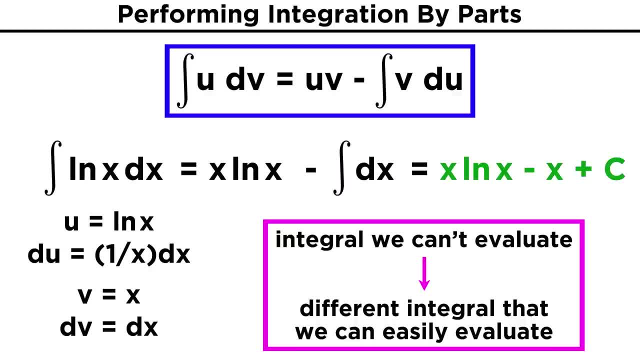 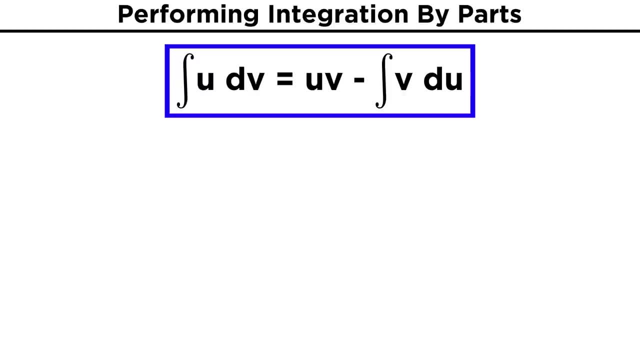 to be much easier to evaluate. This won't always work, but when it does, it certainly is useful. Let's do a few examples that are slightly more difficult, just to make sure we understand. First, let's integrate the natural log of x over x squared dx. 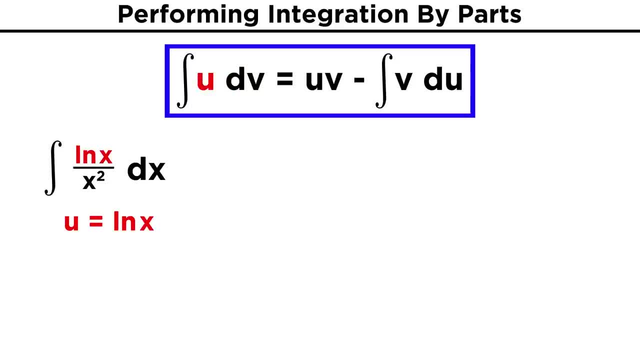 Here we have to choose which is u and which is dv. Let's try natural log of x. Let's try natural log of x for u. So u equals natural log of x and dv is the rest, or dx over x squared. 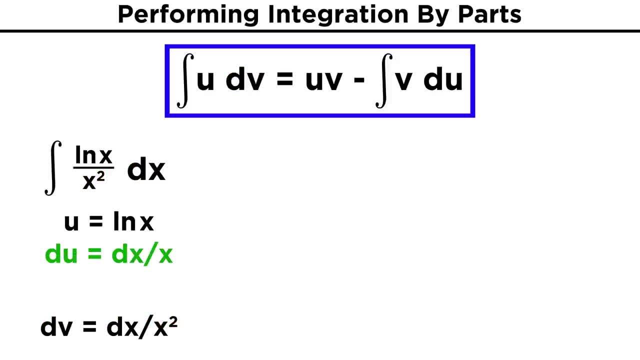 That means du is one over x, dx or dx over x, which does look simpler like we intended. And for v, we realize that integrating x to the negative two gives us x to the negative, one over negative one, which is negative. one over x. 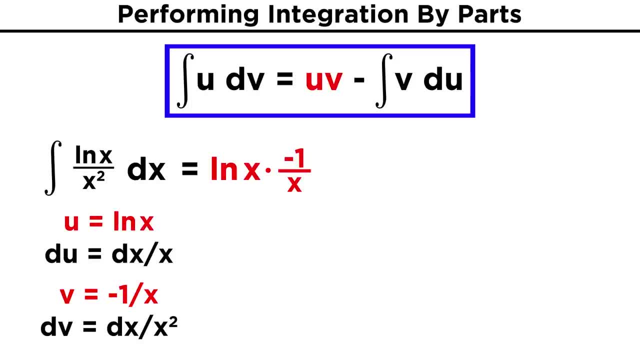 So to evaluate this, we write uv, which here will be lnx times negative, one over x, or negative lnx over x. Then we subtract the integral of vdu, which will be negative one over x times, one over x dx. We can take the negative out to cancel out the first, making this a plus sign. and inside: 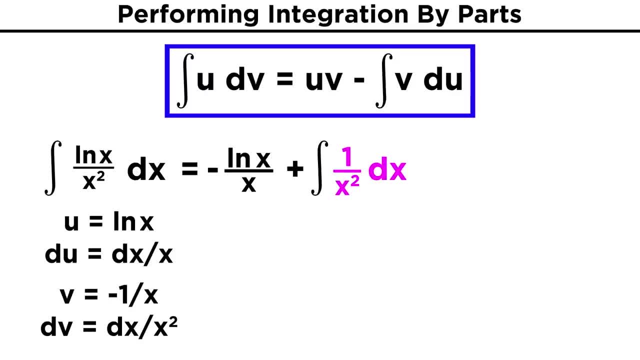 the integral we have one over x squared dx Or x squared dx or x to the negative two dx. We can integrate this to get negative one over x once more. so we end up with negative ln, x over x, minus one over x. 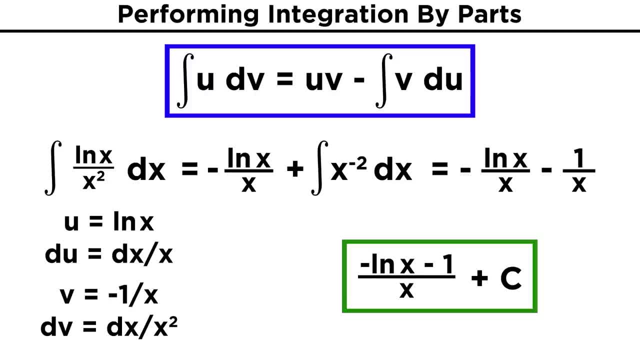 We can combine those fractions and that's the answer, remembering to add plus C, as we always do when dealing with indefinite integrals. It may not look great, but if that's what we get, then that's what it is, no matter. 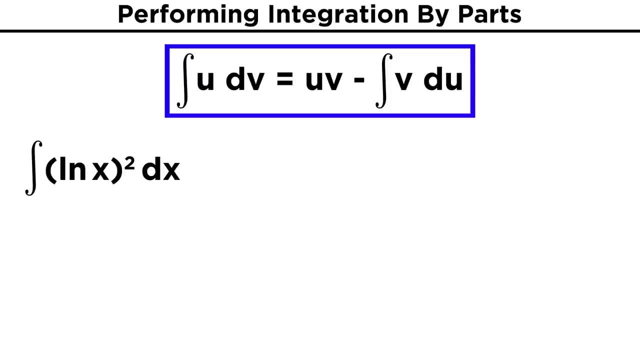 how pretty or ugly. How about one more for good measure? let's evaluate the integral of the natural log of x quantity squared dx. Here we have only one choice: u will be this term and dv will simply be dx. So getting du will require the chain rule and we get two times ln, x times the derivative. 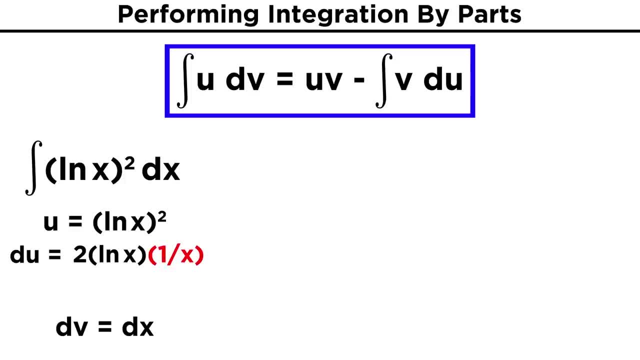 of ln x, which is one over x. So that gives us two ln x. Now we have two ln x over x dx. Getting v is no problem. from dx we just get x. So plugging things in uv will be x times ln x, quantity squared. 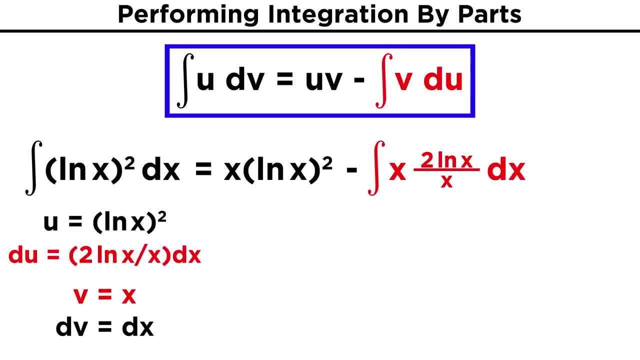 Then we subtract from that the integral of x times two ln x over x, The x's cancel, leaving us with two ln x. Let's take out the two to get simply put dx. Let's take out the two to get simply put dx. 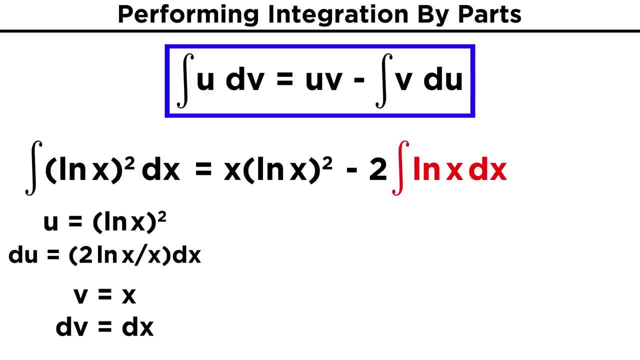 Let's take out the two to get simply put dx. Let's take out the two to get simply ln, x. Well, we can't integrate this normally, but, as we saw in an earlier example, we can integrate this by parts. so we just repeat this process. 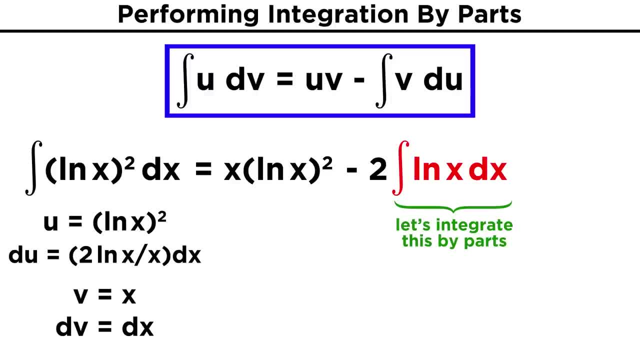 It may seem unfair to have to do this twice, but in performing this technique we produce a new integral, and if that second integral must be integrated by parts, then that's just what we have to do. Let's put some brackets around this integral so that we don't make any careless changes. 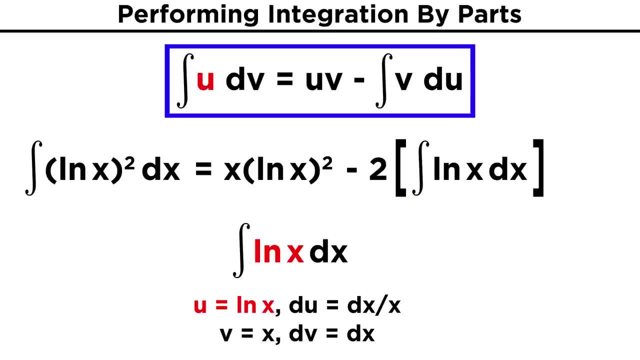 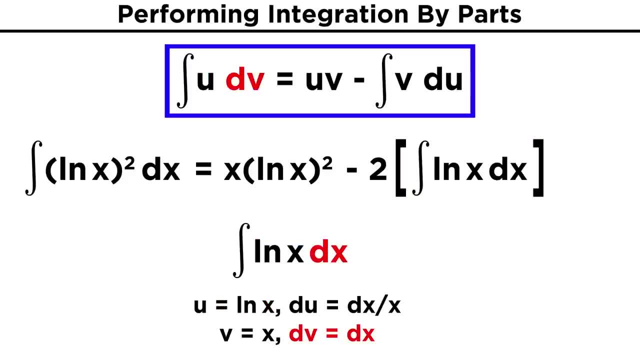 Just as before, u will be ln, x, dv will be dx and that makes du equal to dx over x and v equal to x. So, all still within these brackets, we can rewrite this integral as x, ln, x, minus the integral of dx. 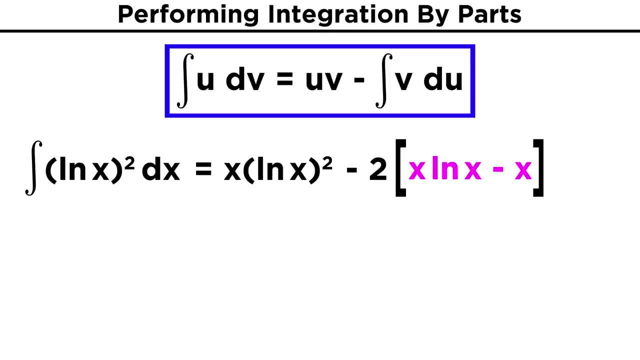 That integral becomes x, so it's x, ln x minus x. That integral becomes x, So it's x ln x minus x. distribute this two from before across this term, which will all together give us x- ln x. quantity squared minus two x, ln. x plus two, x plus C. 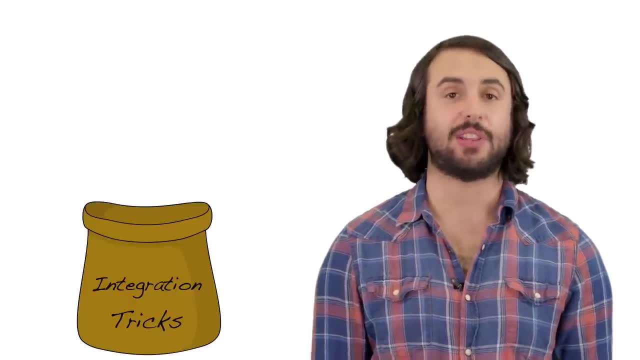 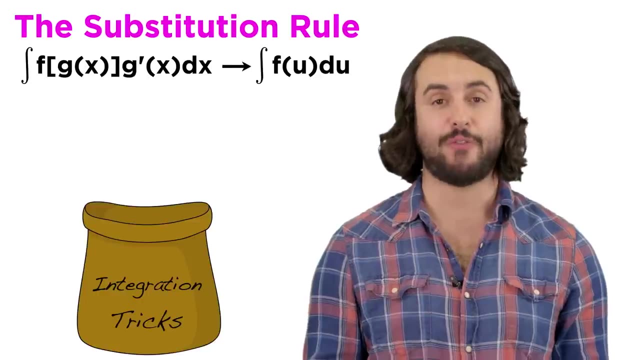 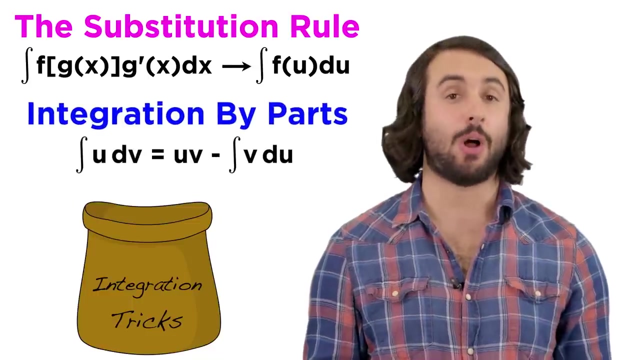 So integration by parts is just another technique in our bag of tricks that we can use to evaluate integrals. The substitution rule works well when the integrand is the product of a function and its derivative or close to it. Integration by parts works when the two functions are not related at all, but one of them becomes. 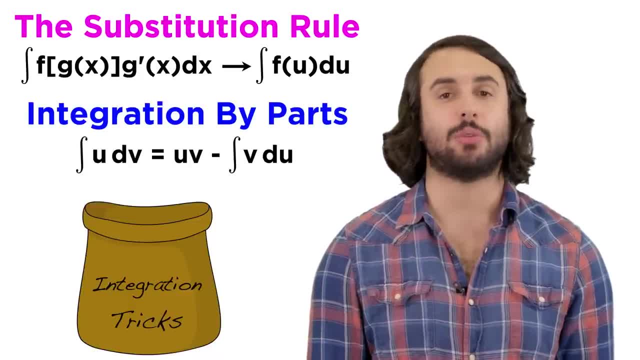 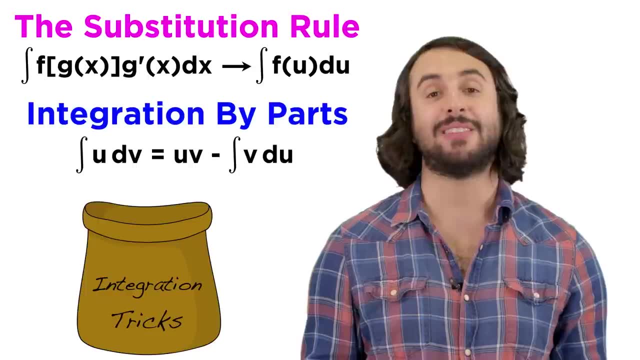 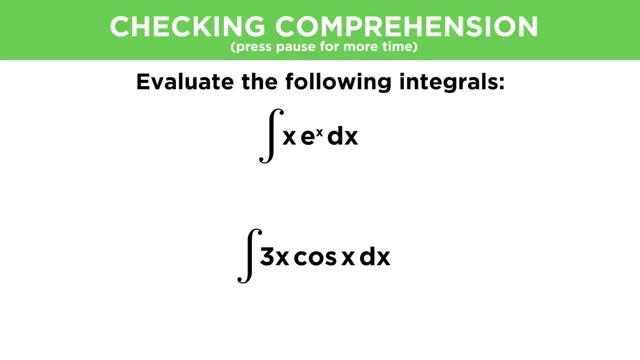 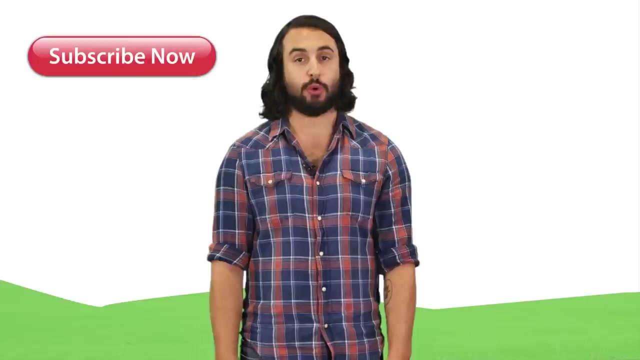 much simpler when differentiated, which makes the new integral easier to solve than the original one. We have one more trick to learn regarding integration, but before we move on to that, let's check comprehension. Thanks for watching, guys. Subscribe to my channel for more tutorials. 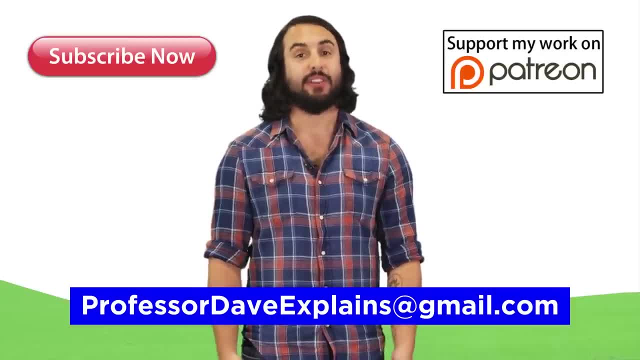 Support me on Patreon so I can keep making content and, as always, feel free to email me. I'm jamesplains at gmailcom.